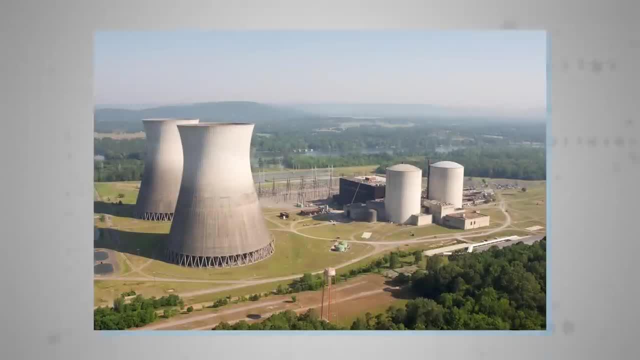 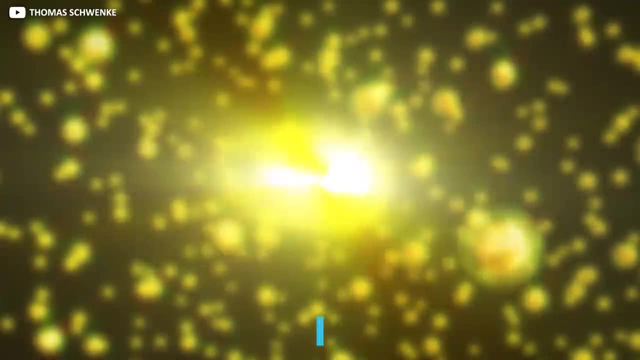 survive. It could also be used to produce carbon-fumed or stubbornly indestructible radioactive waste generated by other less-efficient means of power generation. So how does nuclear fusion work? Conventional nuclear power plants rely on the process known as nuclear fission In a 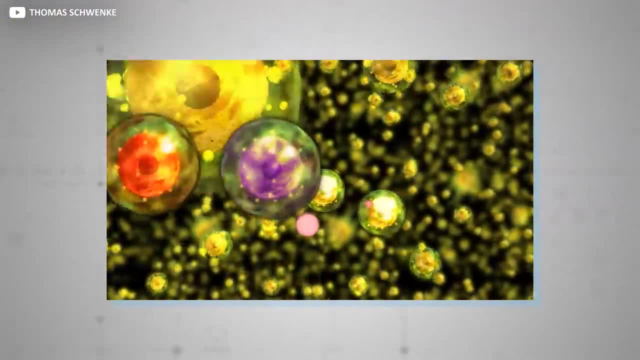 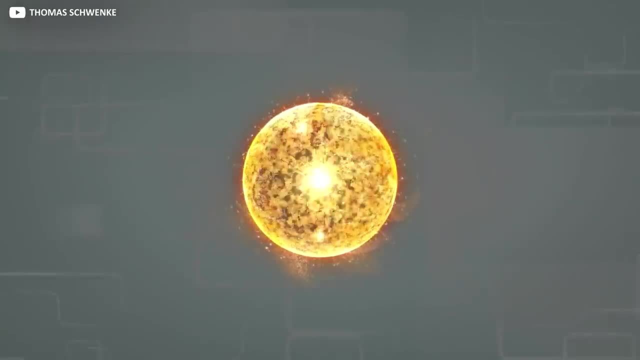 fission reactor, stray neutrons slam into larger atoms, typically uranium or plutonium, causing them to split. This in turn releases energy and even more neutrons, which go on to split still more atoms, causing that dramatic chain reaction we're all familiar with from 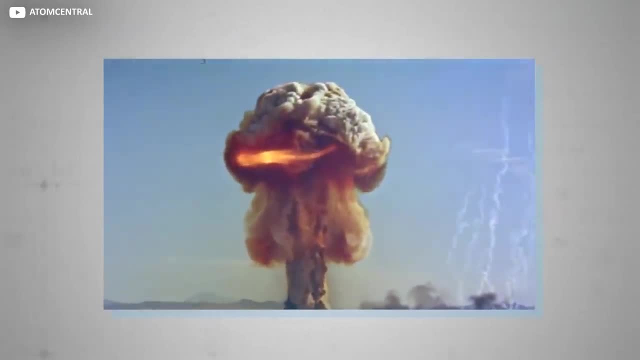 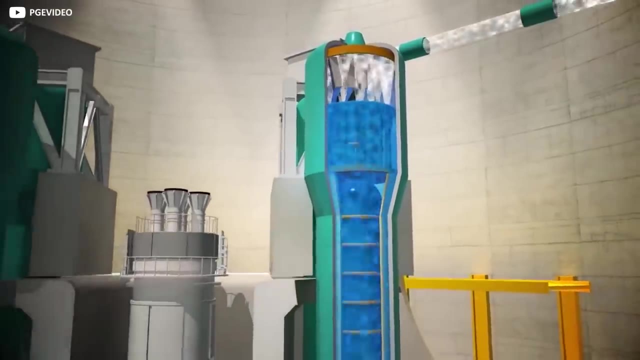 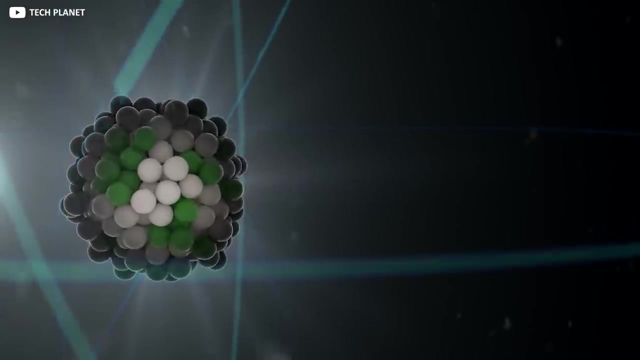 disaster movies and terrifying old-school footage of ginormous bombs going off. In a regular nuclear power plant, the heat generated by that runaway reaction boils water, which generates steam that in turn drives turbines in order to create electricity. Fusion, even though the word sounds inconveniently similar to fission, is a different process. 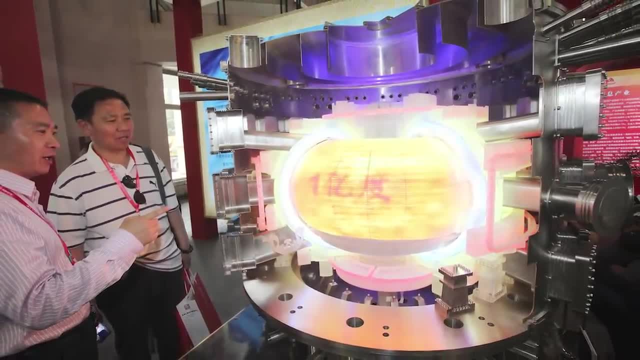 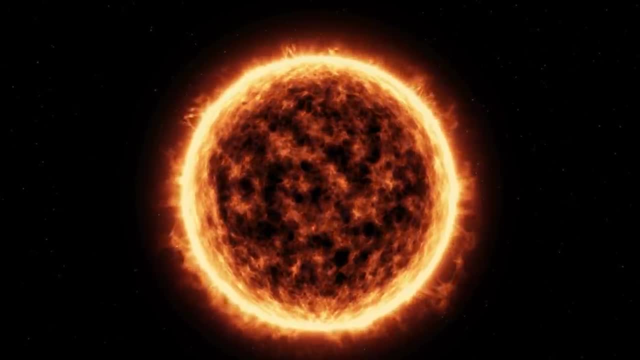 altogether. In a fusion reactor, two or more lighter elements, typically isotopes of hydrogen, are smooshed together to form a larger element, usually helium. This is exactly the same chemical reaction taking place right now in the heart of every star. Fusion is capable of producing. 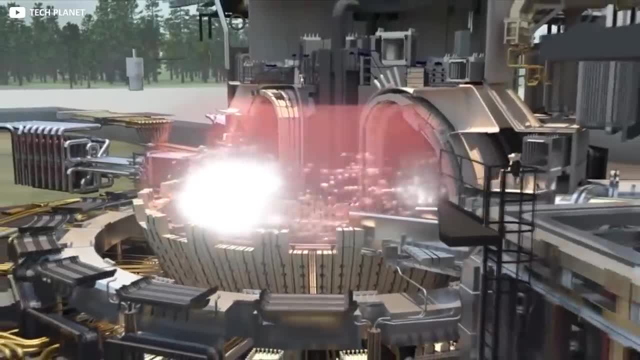 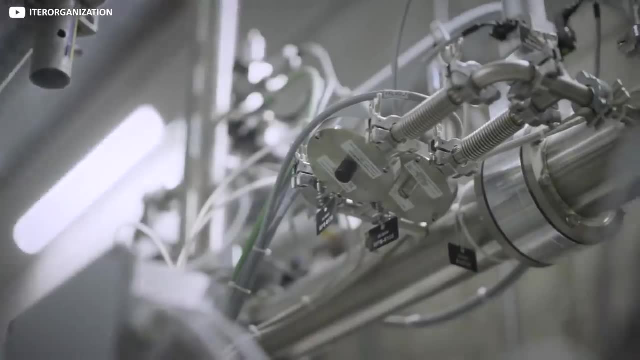 times as much energy as fission, not to mention many millions of times the energy generated by grubby, old-fashioned fossil fuels. You might reasonably ask at this point why every nuclear power station isn't already fusion-based. Well, for fusion to take place, three very difficult conditions need to be. 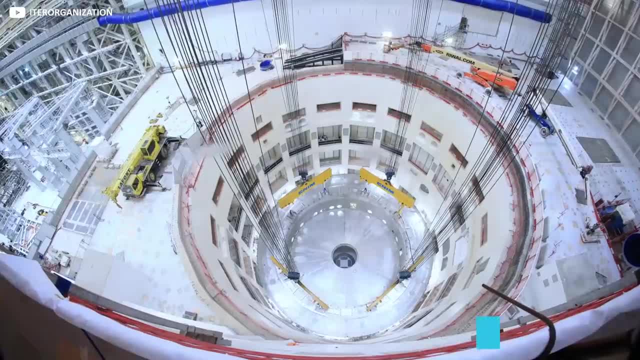 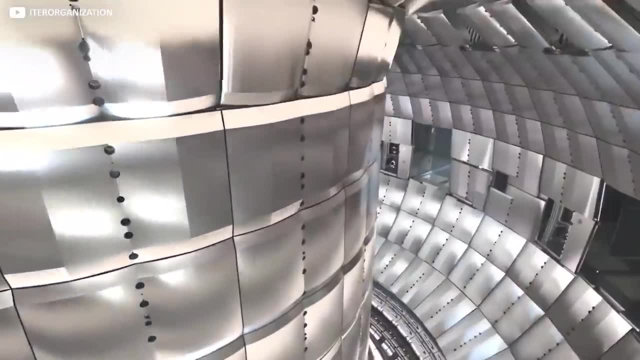 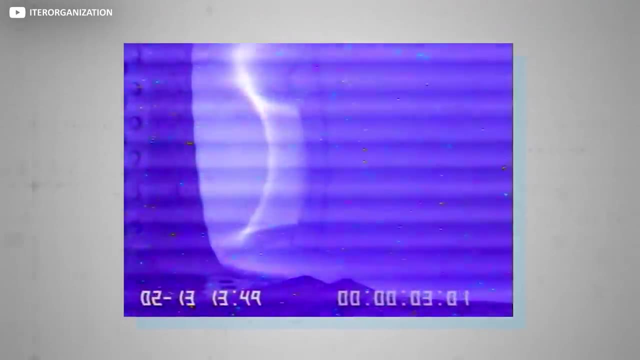 met. First, the temperature in the reactor core needs raising to around 150 million degrees Celsius before fusion can even theoretically take place. That's quite an energy-intensive process in itself. Secondly, the so-called plasma in which this reaction occurs needs to be of sufficient density to make fusion a likelihood. And third, 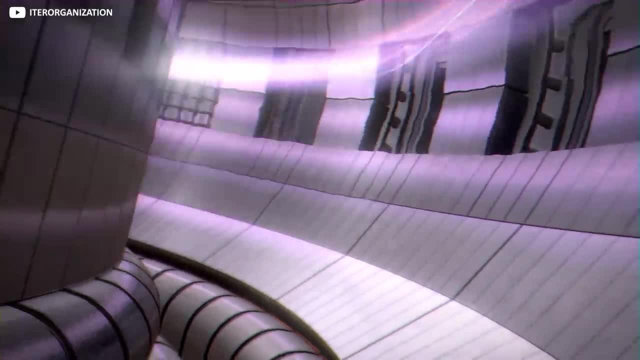 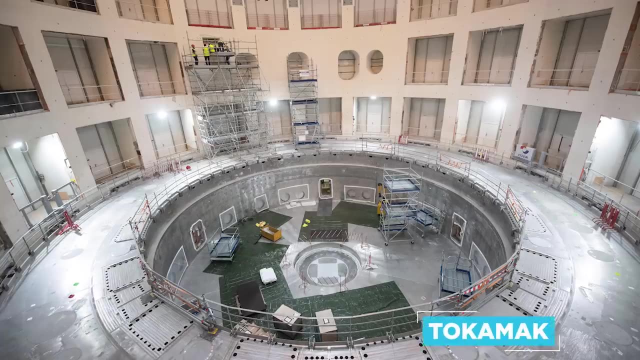 this plasma needs to be held in confinement for long enough for the power generated to be usefully harnessed. To this end, ITER engineers are presently assembling a gigantic structure known as a tokamak. This contraption was first proposed by Soviet nuclear physicist Igor Golovin back. 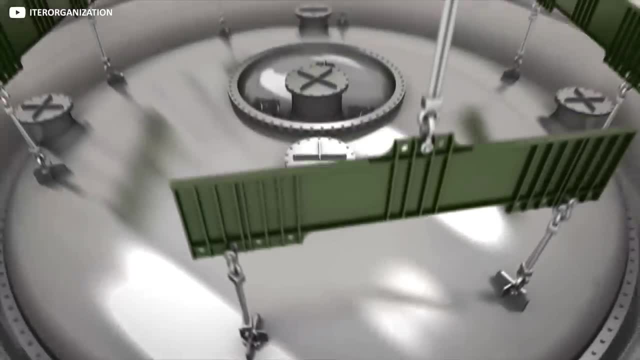 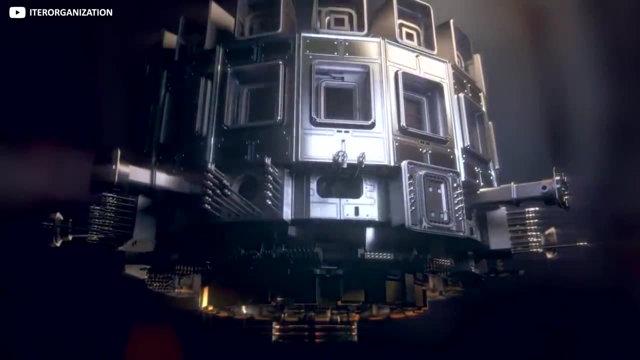 in 1957.. Tokamak, which, since you ask, is a Russian acronym meaning toroidal chamber with magnetic coils, is essentially a vast steel doughnut where ultra-strong magnets conspire to create sufficient heat and pressure in a vacuum to turn gaseous. 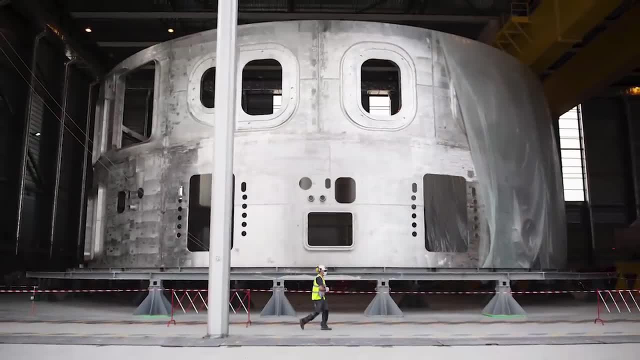 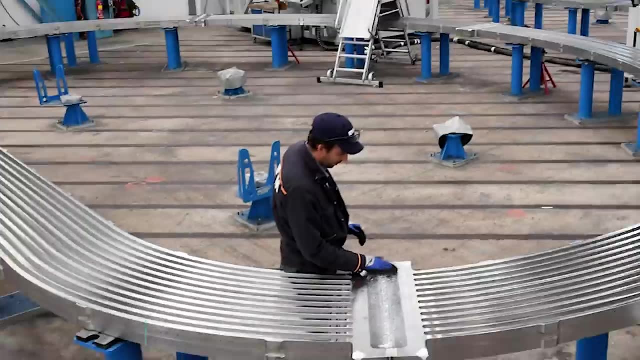 hydrogen fuel into a plasma. The tokamak at ITER is by far the largest ever constructed. Each one of its 18 D-shaped toroidal field coils – huge magnets in essence – weigh 310 tons, or about the same as a fully-laden jumbo jet. That's before we get to its six. 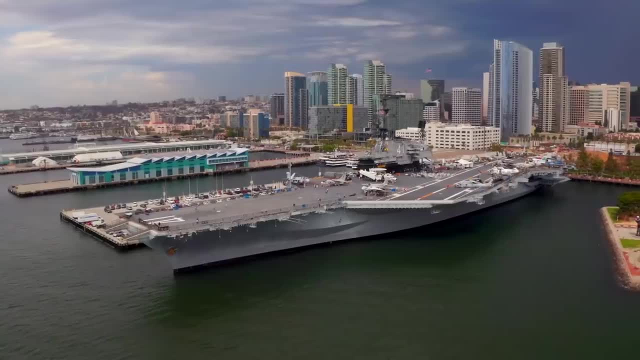 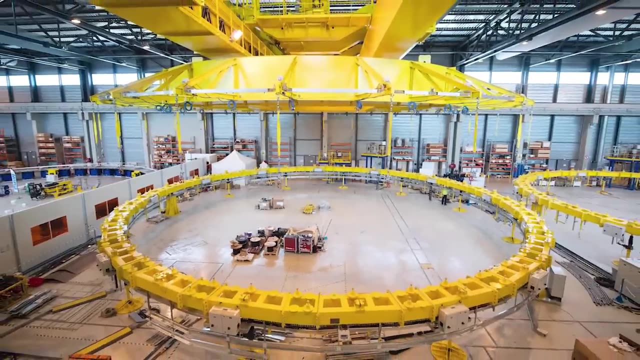 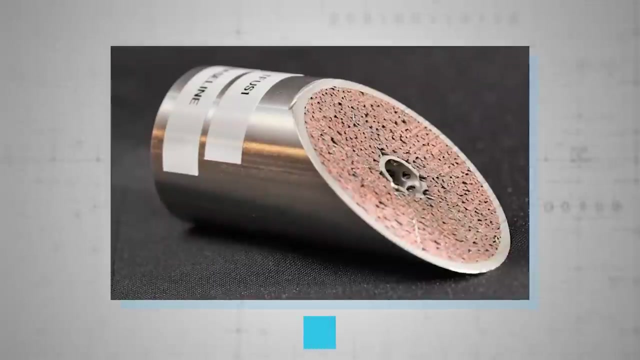 poloidal magnets and this colossal central solenoid that's theoretically strong enough to lift up an aircraft carrier. All this in a tokamak chamber that's twice the size and ten times the internal volume of anything previously attempted To keep the largest superconducting magnet system ever running through a hundred-thousand. 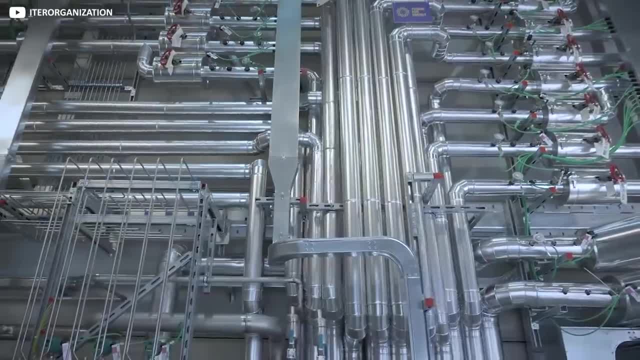 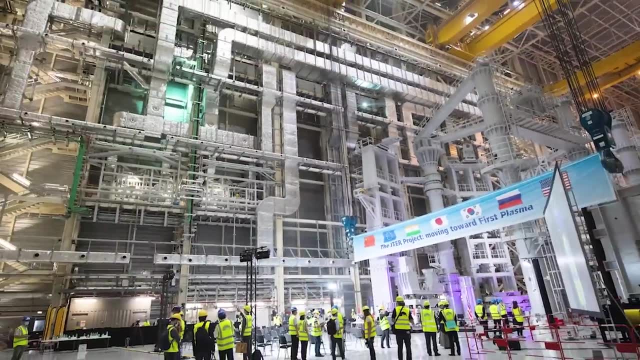 kilometers of niobium-10 superconducting wires. the world's largest helium refrigeration unit is being manufactured at the same time. To put all that in perspective, when it's finished, the ITER facility will be home to both one of the hottest places in the universe. – 150 million degrees Celsius in the reactor chamber – and one of the coldest places in the universe: 69 degrees C or 4 Kelvins in the coolant system. As if summoning the power of a literal star wasn't tricky enough, ITER also happens. 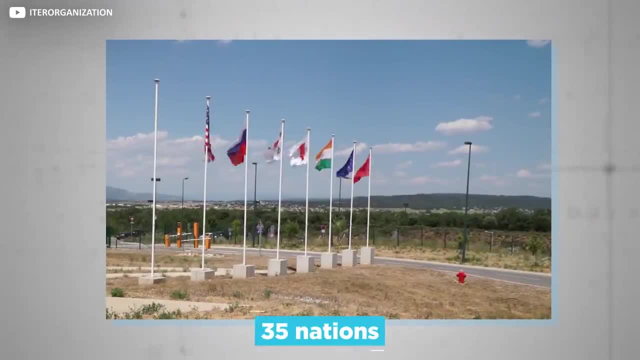 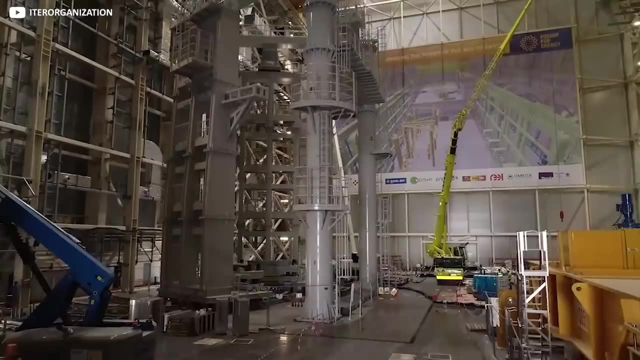 to be a complex collaborative effort between some 35 nations, each assembling their own parts to be assembled on site. As you might expect, this presents some tricky logistical challenges. Certain individual components among the estimated 10 million parts that will go into ITER are: 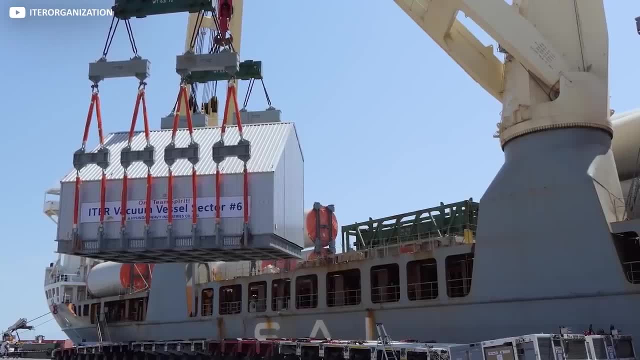 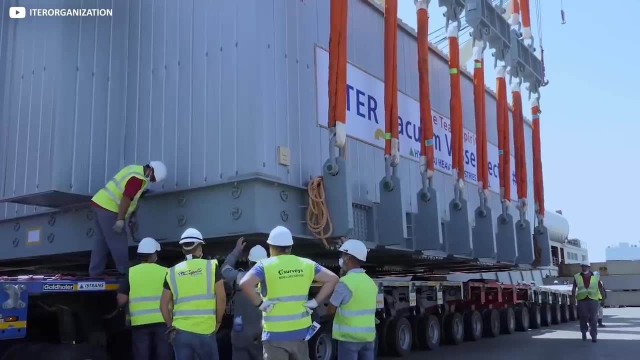 being shipped from as far away as South Korea. Some bits weigh 900 tonnes and others are four storeys high. A 104-kilometre road from ITER's nearest Mediterranean port, at Fos-sur-Mer, near Marseille, has been specially upgraded at eye-watering cost. 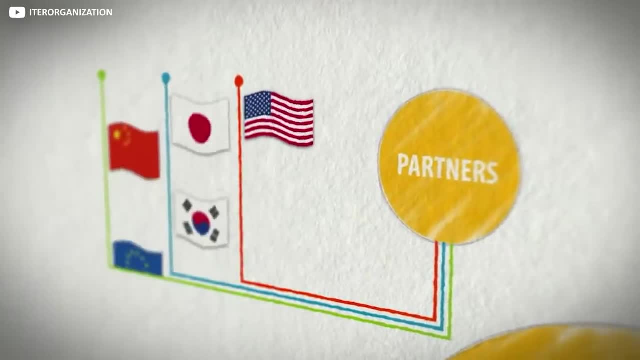 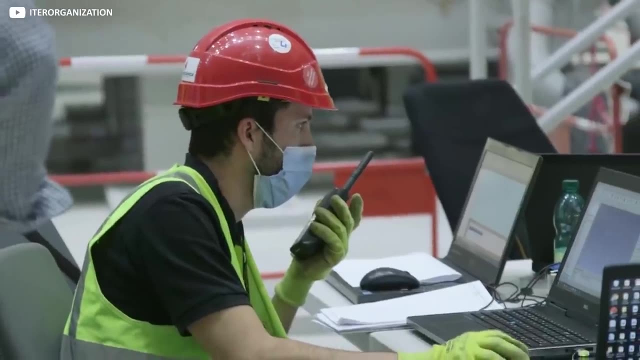 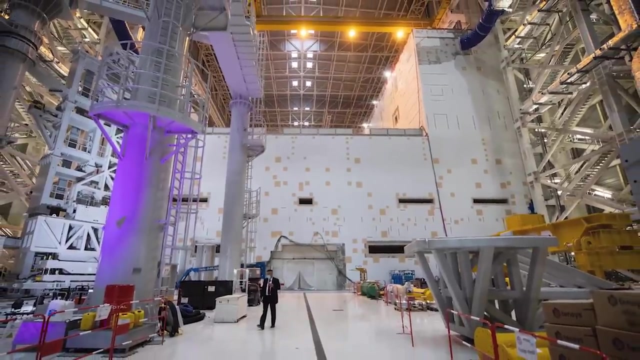 This multinational endeavour, which takes input from the European Union, United States, Russia, China and India, among others, promises stakeholders, in exchange for their support, priceless experimental data and access to any intellectual property generated as a consequence of the project, When ITER finally manages to assemble this enormous, fiendishly complex jigsaw puzzle. 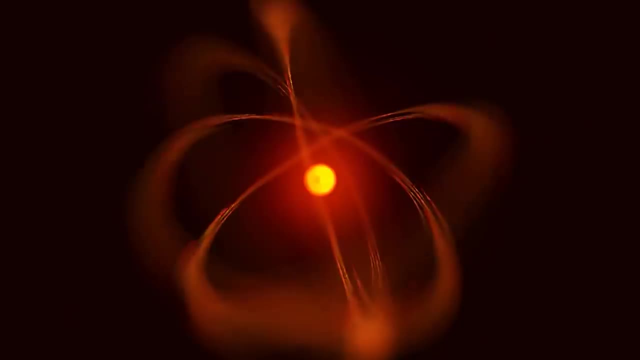 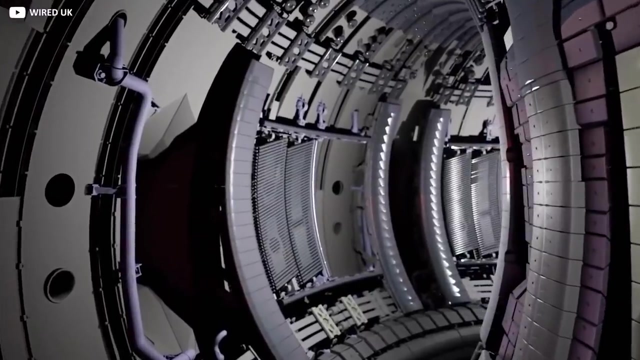 the project has fun Five concrete aims. The first is to produce 500 megawatts of power from a fusion reaction. So far, the record is just 16 megawatts, held by another smaller tokamak known as JET in. 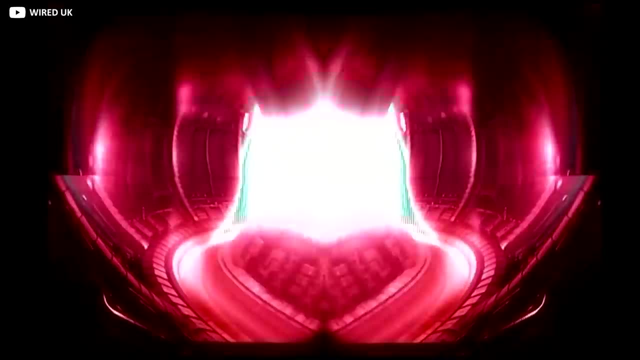 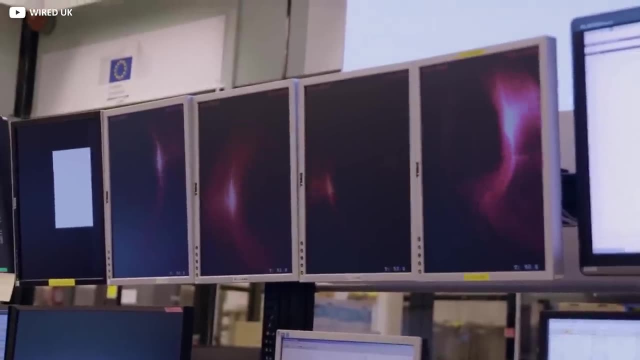 Cullum, England, which achieved this benchmark back in the 1990s. However, the JET team required 24 megawatts of heating power to even manage this. In essence, a net loss of 8 megawatts. 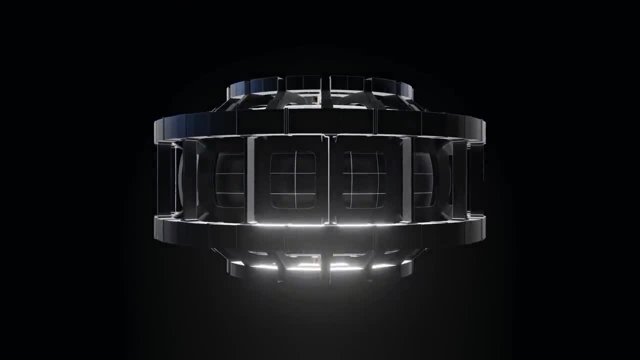 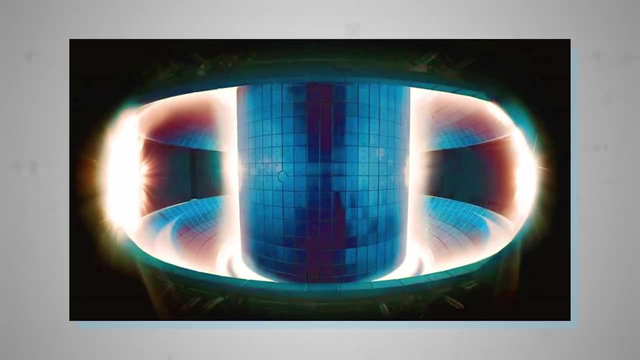 At ITER. the plan is to use associated techniques to raise the temperature inside the reactor to 150 million degrees C And hope its plasma achieves a sustainable burn from a mere 50 megawatts of input heating power. If they pull that off, it will be the first time fusion has ever generated more power. 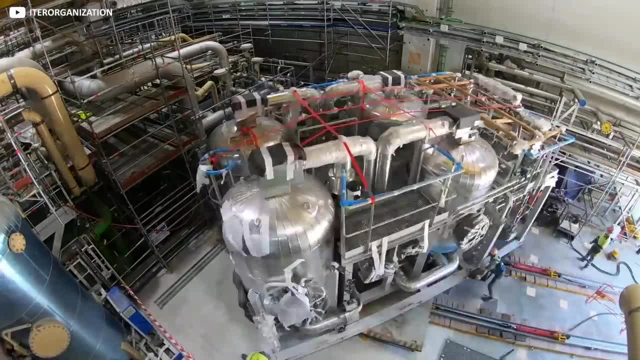 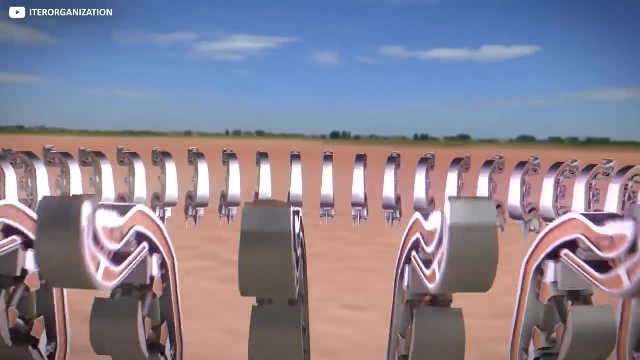 than was put in by a healthy factor of 10.. The second target for ITER is to demonstrate feasibility for the myriad associated technologies needed to support a fusion reactor. That means heating the tokamak's elaborate diagnostic systems, its vast cryogenic apparatus. 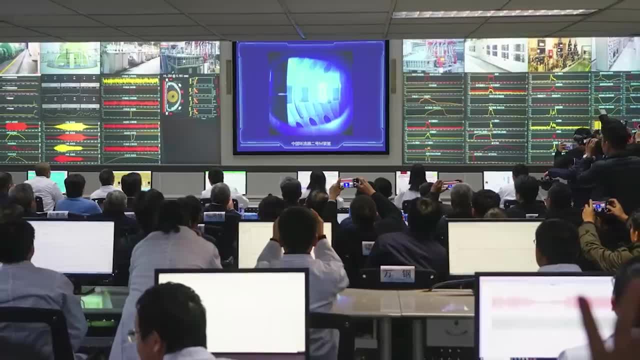 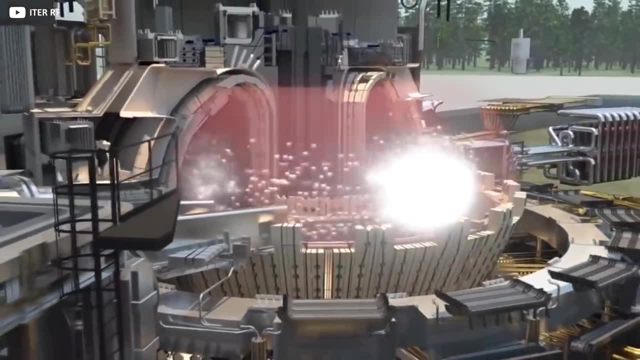 for keeping the magnets cool and everyday boring stuff like maintenance and control systems. ITER's third aim is attaining the holy grail of so-called burning plasma. that is, a fusion reaction which generates its own heat, making it sustainable for longer periods than is. 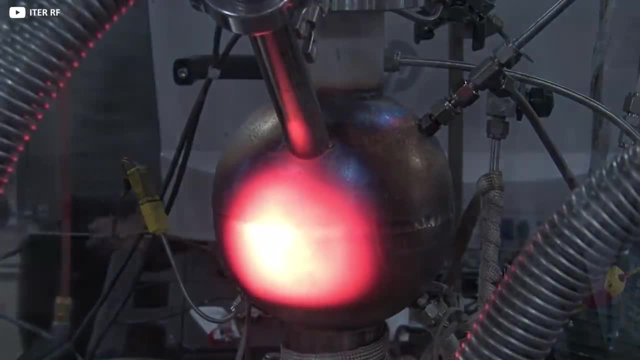 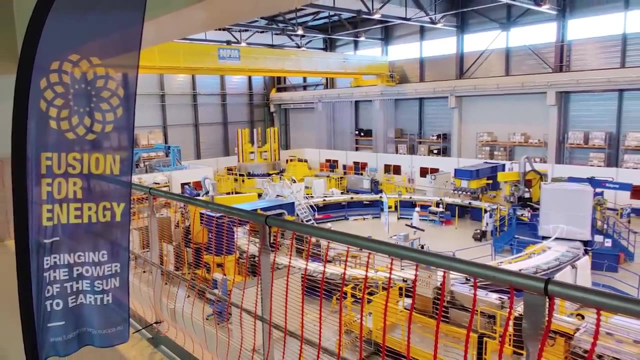 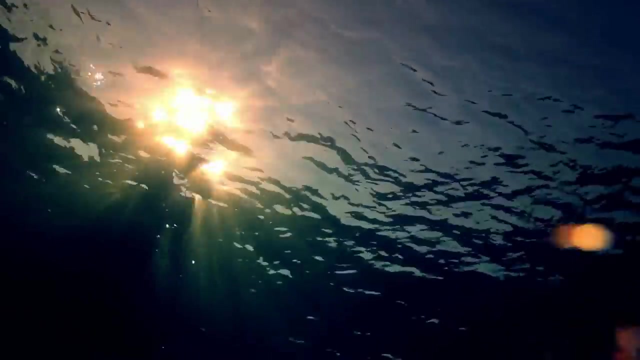 currently possible. The fourth target is arguably the most important: to prove the feasibility of so-called tritium breeding. It was established long ago that the most likely fuel for dependable fusion reactions is a cocktail of deuterium and tritium. Deuterium is, as luck would have it, super abundant, occurring naturally in seawater. 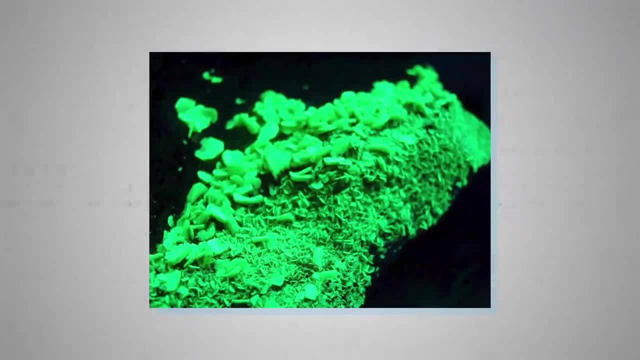 Tritium, on the other hand, is extraordinarily abundant. It is the most likely fuel for dependable fusion reactions. Tritium, on the other hand, is extraordinarily scarce, with only around 3.5 kilograms at any one time available in nature- nowhere near enough to fuel that hoped-for fusion energy. 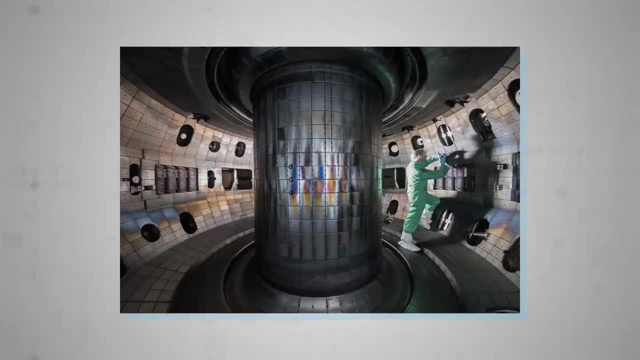 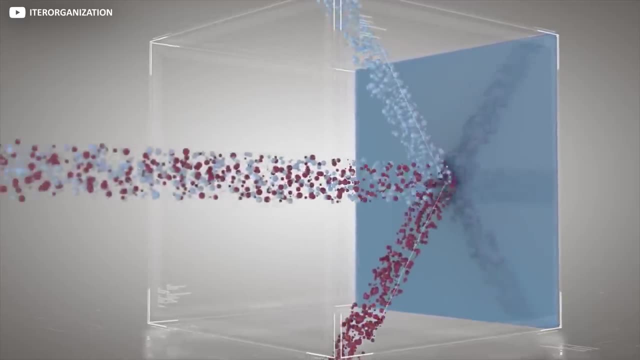 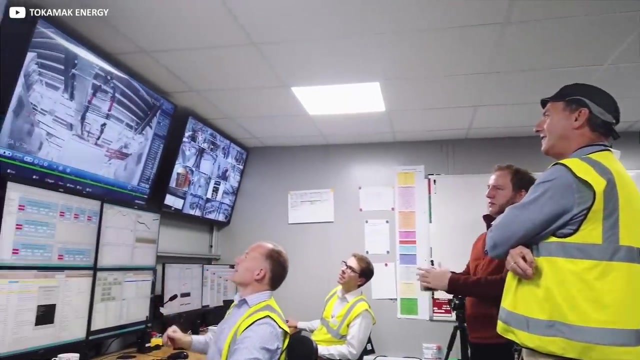 boom. As such clever ITER engineers have lined their reactor wall with a nifty breeding blanket comprising lithium-based materials in order to hopefully harvest and generate tritium as a by-product of the fusion reaction itself. The fifth and final target for ITER is, of course, to prove the safety of a fusion device. 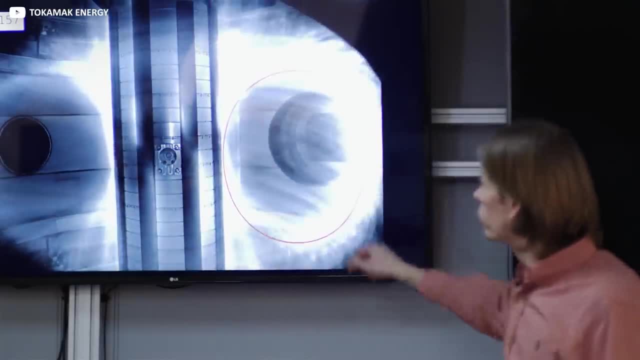 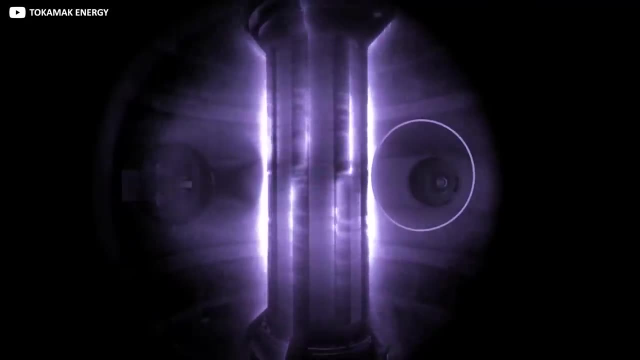 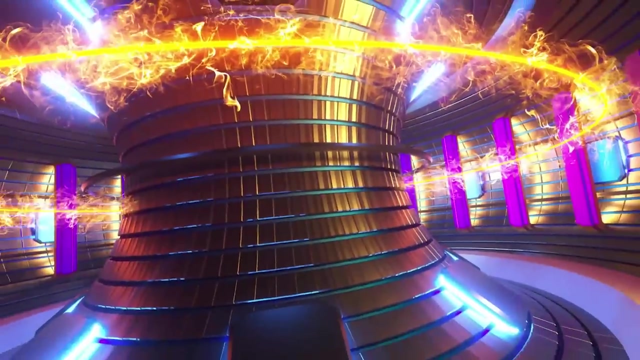 which is a must in a world of vocal nuclear energy sceptics. After many years of delays and changes in senior personnel, the ITER project is finally in the construction stage and expects to fire up its first plasma in December of 2025.. If all goes to plan, three processors will work in concert to raise the core temperature. 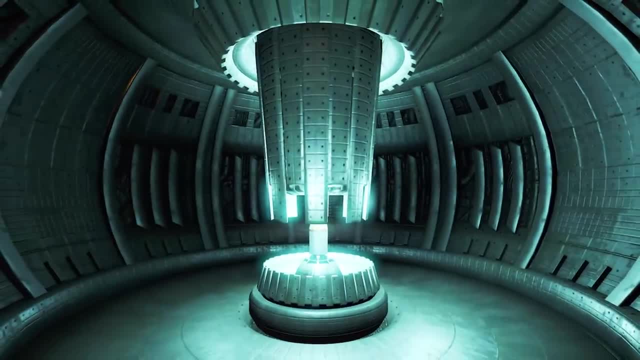 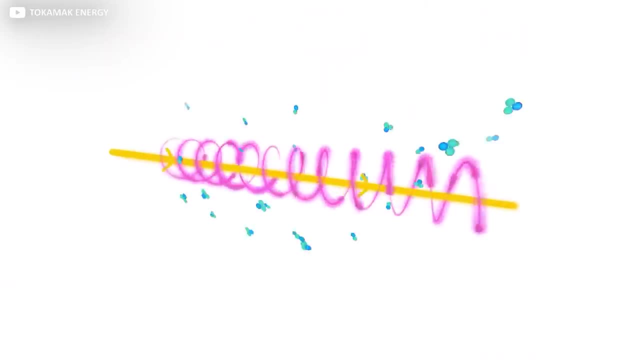 to the magic 150 million degrees C necessary for fusion to occur. These are ohmic heating, created by smart manipulation of those mighty magnetic fields, neutral beam injection of high-velocity charged deuterium and high-frequency electromagnetic waves, a bit like your microwave at home.